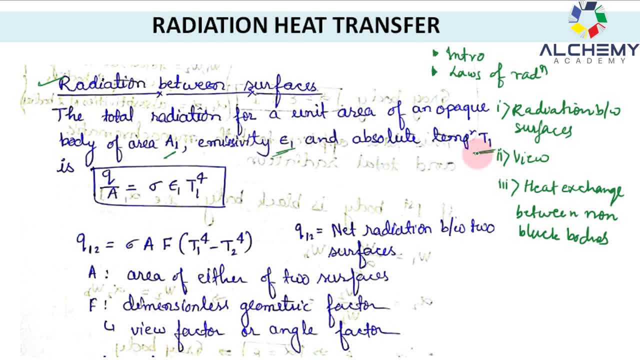 Emissivity, epsilon 1 and the absolute temperature, T1 is given as Q by A is equal to sigma, into epsilon, into T1 raised to the power 4.. If it is a black body, then emissivity, your emissivity, will be 1.. 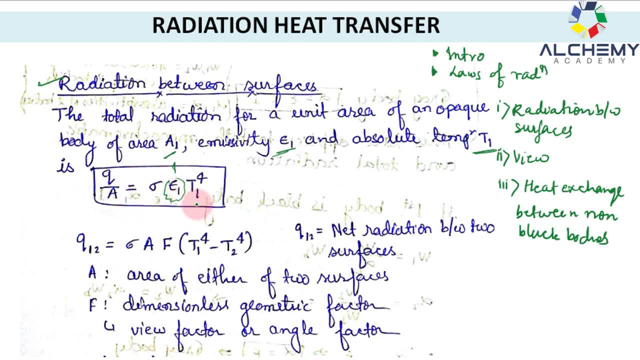 So it becomes Q by A is equal to sigma into T1, raised to the power 4.. So it is kind of Stefan Boltzmann law. So here there is a emissivity factor E1. So Q12.. Q12 is basically the radiation net radiation between the two surfaces. 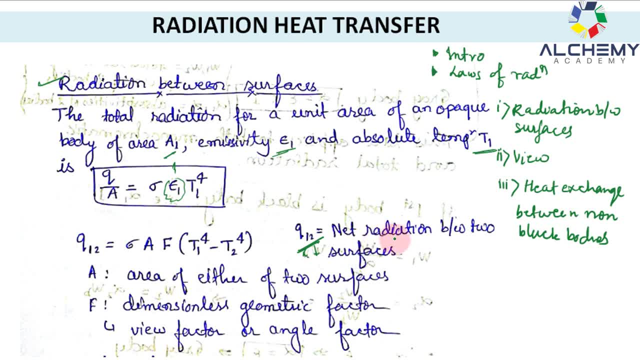 One is surface 1, two is surface 2.. So this is net radiation between two surfaces. So it becomes sigma into A, into F, into T1 raised to the power 4 minus T2 raised to the power 4.. So we must know about the factor F. 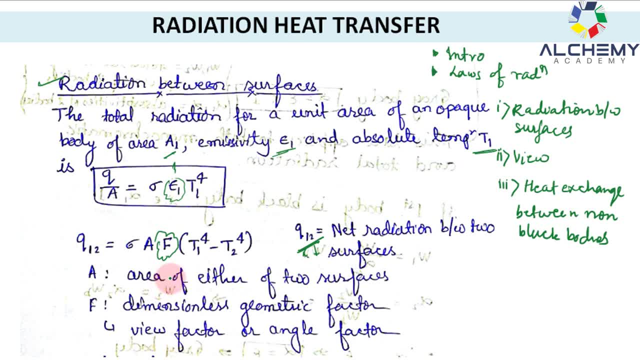 It plays a very important role. So here is area of either of the two surfaces. Suppose two surfaces are there. Either it can be parallel surface or one body surrounded by another body. Okay, So any dimensions we can consider. So area of either of the two surfaces. 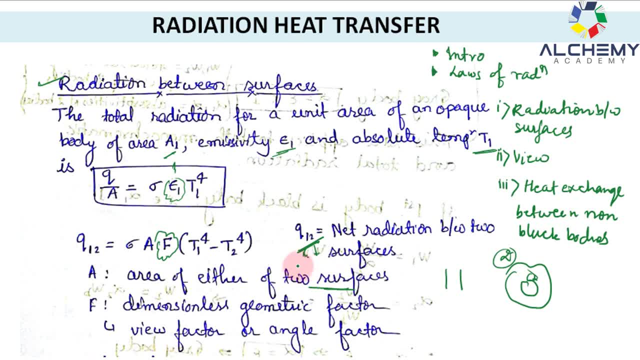 So either first surface, area of first surface or area of second surface. We can write in terms of anyone. We can write in my next slide: And F is your dimensionless geometric factor. It is also called as a view factor or it is called as angle factor. 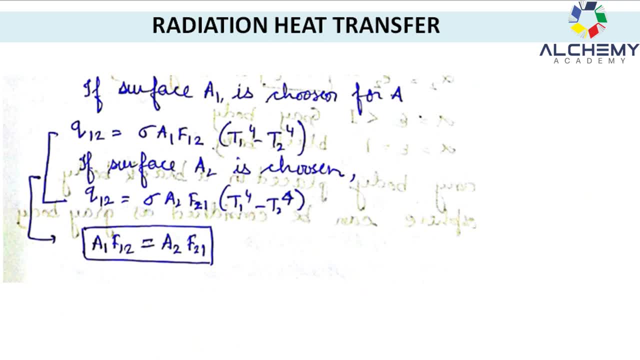 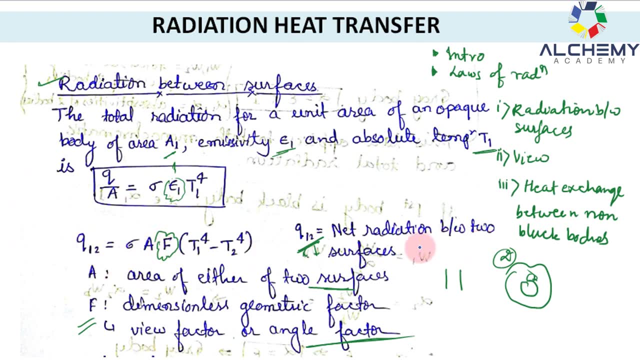 Now, if we are going to write that net heat exchange, This Q12 net radiation between two surfaces in terms of area A1. Then what happens This? your A becomes A1. And then F become. it becomes F of 12 means What is view factor F of 12?? 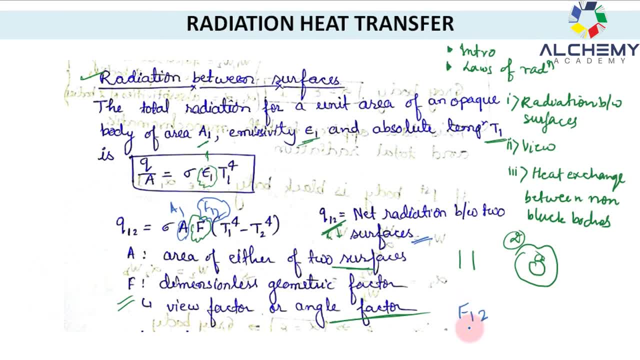 It is basically, if it is written as 1 and 2.. So one is considered as source- Source means the source from where radiation is getting emitted, and two is your receiver. This is called as a receiver amount of energy that has been intercepted by bodies to. 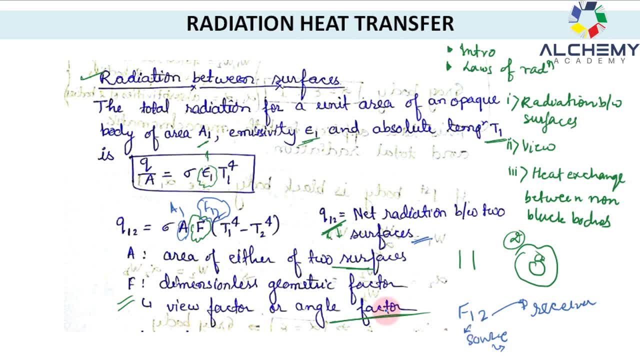 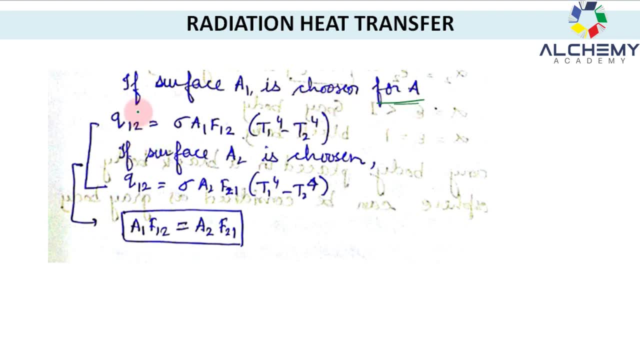 From bodies radiation emitted by the body one. So if surface A1 is chosen for A, that is it is. we can write, as Q of 12 is equal to Sigma, into A1, into F of 12, into, in bracket, T1 raised to the power, 4 minus T2 raised to the power. 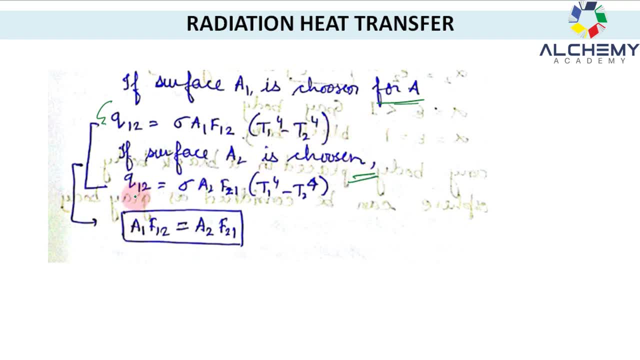 4. So if surface A2 is chosen, we can write as Q of 12, as Sigma, into A2, into F of 12, into T1 raised to the power 4.. So F12, F12 means amount of radiation intercepted by body to, that is, that has been emitted by. 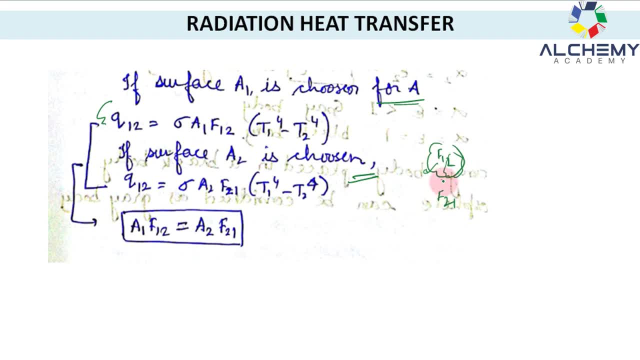 body one, Whereas F of 21 is vice versa of F of 12.. So if we equate these two, Q12, because net radiation exchange between two bodies. If you write between body one or body two, or you can say as body two or body one, since 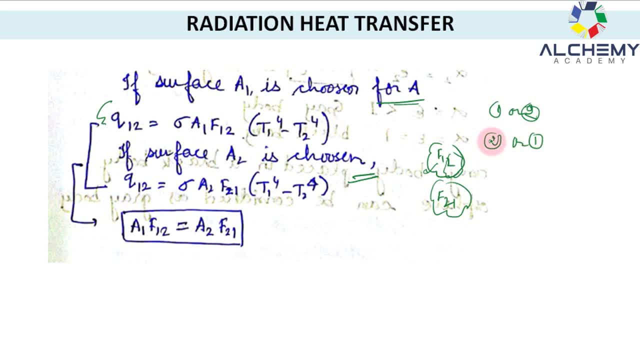 bodies. only two bodies are there. So what happens? net radiation exchange between these two parties bodies will be would be same whether you write in terms of Q12 or you write in terms of like, you write in terms of F of 12, area one, or if you write in terms of area A2.. 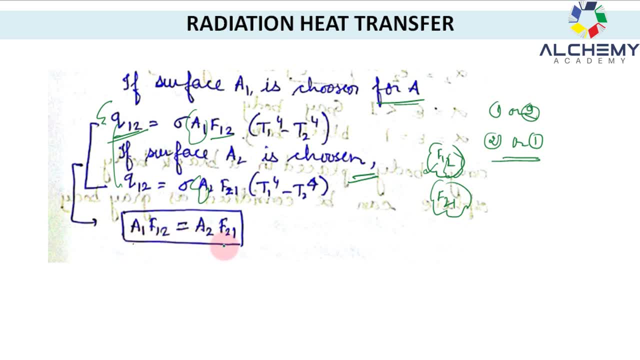 So if you equate these two will get A1. F of 12 is equal to A2 into F of 21 means a view factor. area of one body is given and view factor of this body is given. and suppose area of second body is not given but view factor is given, then we can calculate the area two. 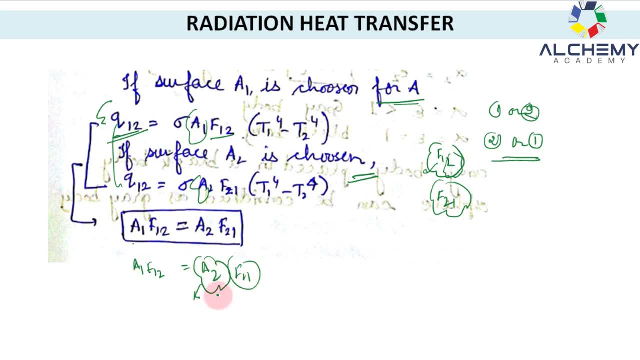 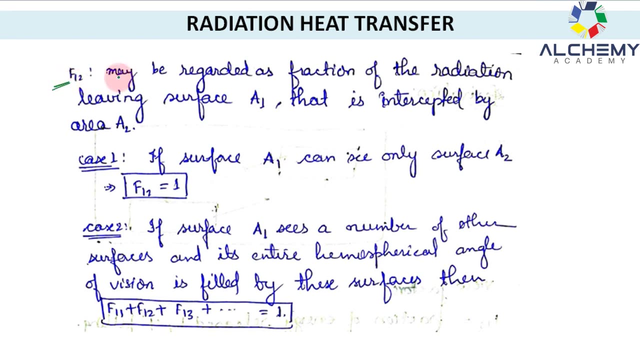 but in case, if area two is given, a view factor is not given, then we can. we can calculate as view factor for the bodies too. So this is the numerical part we can think of now. So F12 is that's what I have told you earlier. F12 may be regarded as fraction of the radiation. 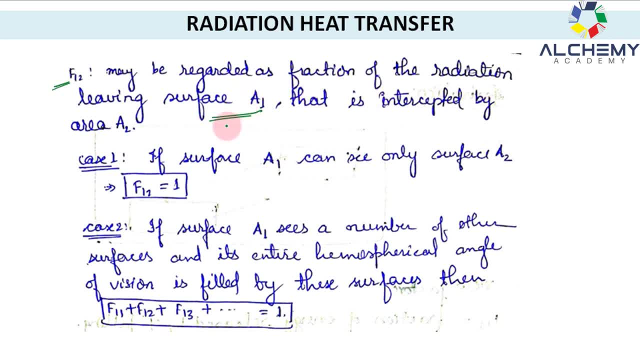 leaving surface even Means fraction of radiation that is leaving surface. even So, how much amount of like anybody, how much amount a body can leave a surface? suppose there is a body radiation incident on the surface, then there is a property, that part of this radiation being reflected. 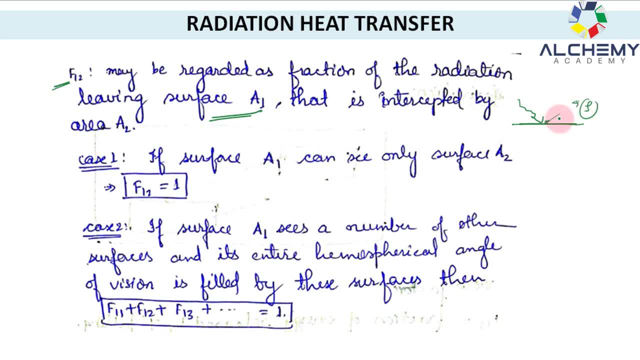 So there is a reflection rho will rho will be taking a, you know, important role here. and the second is there is a tendency of each body to emit the radiation. Okay, So emission part plus the reflected part of the reflected part of the radiation, Okay, 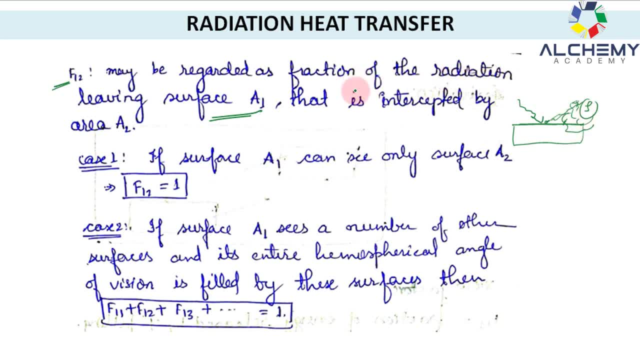 So that is basically your fraction of the radiation leaving the surface, even that is intercepted by body A2.. So fraction of radiation that has been emitted by body one and that is being intercepted by body two. So this is called F of 12 means one. what is one here? one is your source and two is your. 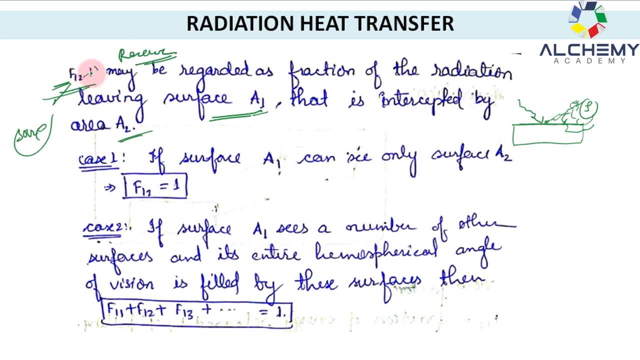 receiver, It is basically the body. Two is basically the receiver as the body which actually indicates that it receives the part of radiation, and one is your basically source that emits the part of radiation. Now let us case one where, if surface A1 can be, only see a surface A2.. 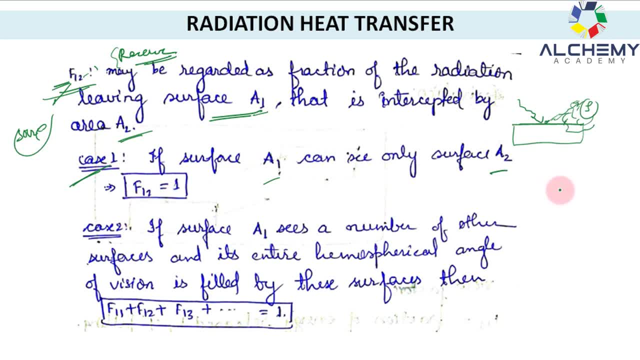 What if surface A1 only see a surface A2? Means, what happens? suppose a body, one body is there and it is one body, this sees only body two. What happens, whatever the amount of energy that is being, you know, leaving the surface one because it sees the surface two only? 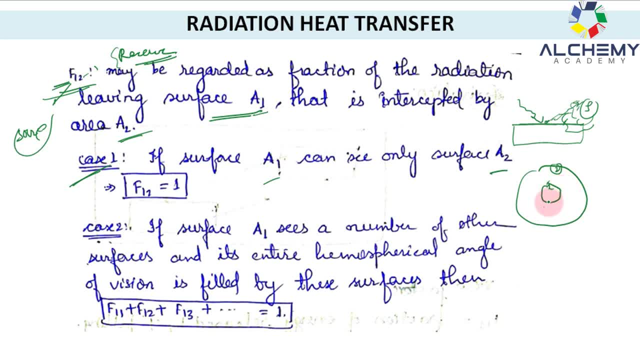 So all amount of you know, the radiation which leaves the surface one will be, you know, intercepted by body two. So in that case, F of 12 would be one. Now let us take a case two, in which, if surface A1 sees a number of other surfaces and its 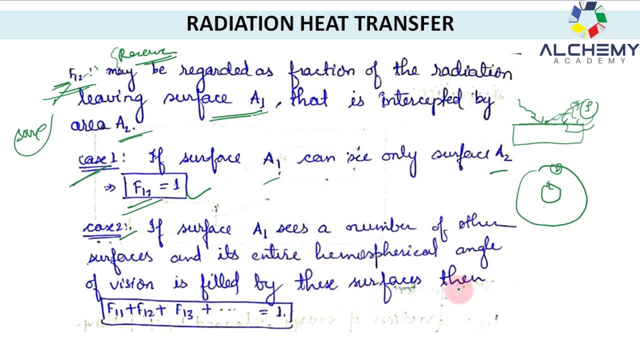 entire hemispherical angle of vision is filled by the surfaces. these surfaces then, in that case, F of one, F of 12 plus F of 13 plus plus dash dash, whatever the number of you know F of one and whatever the number of you know you know, other surfaces are there. 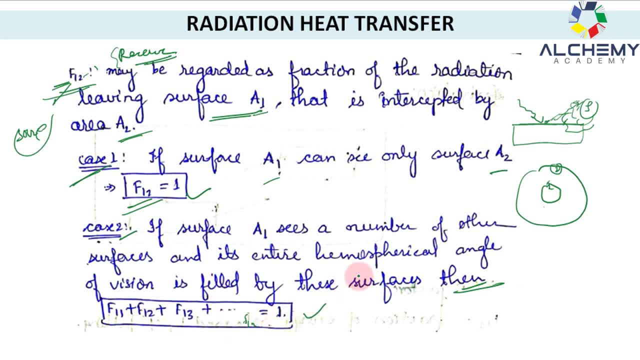 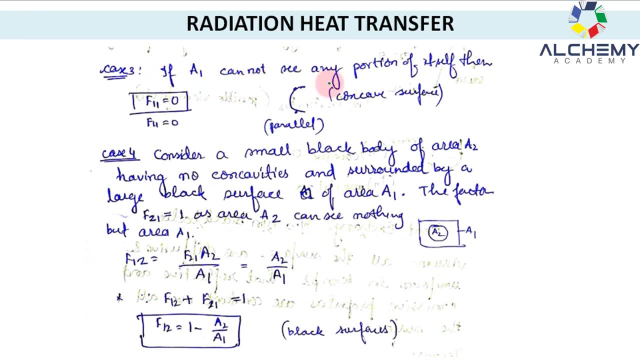 So the sum of all these becomes, you know, considered as one. Now case three: if A1 cannot see any portion of itself, Suppose body one is there. Now, if it is a straight line, okay, If it is a straight parallel surface, any plane surface, then what happens? it won't be able. 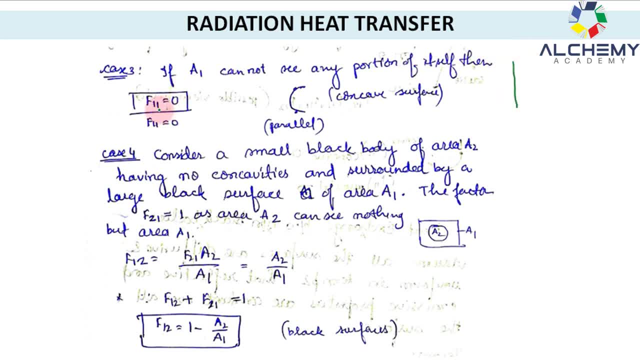 to see his own surface, then in that case one is your source and two is your receiver, part of energy that is leaving the surface. one radiation will not be, you know, intercepted by one because it is a parallel line. So in that case F of one would be zero. 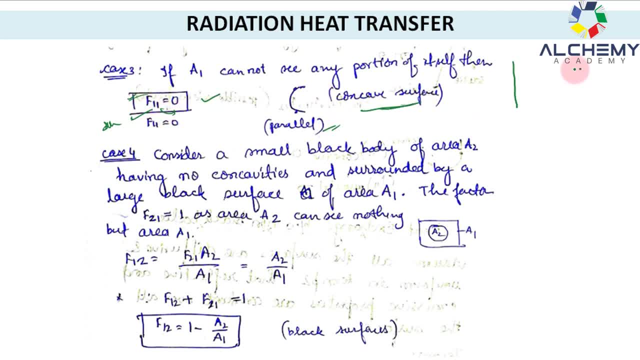 Parallel lines are. it can be concave surface. suppose your surface is like this. any point on this will not be able to see its own part, outer part, Correct. So for these kind of bodies F of one would be zero. Now case four: consider a small black body of area A2 having no con cavities and surrounded 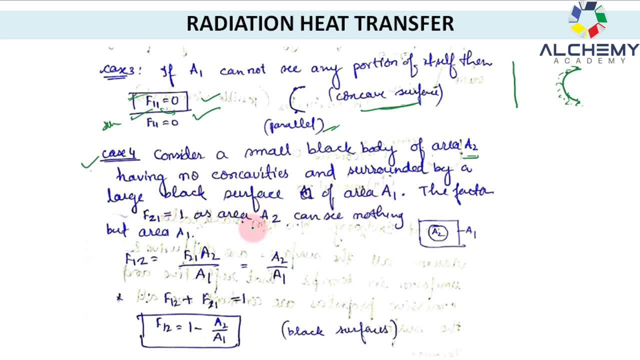 by a large black surface of area A1. The factor F of one, The factor F of two, one is one as area, The factor F of two, one as one, as area A2 can see nothing but area A1. Here is the case. 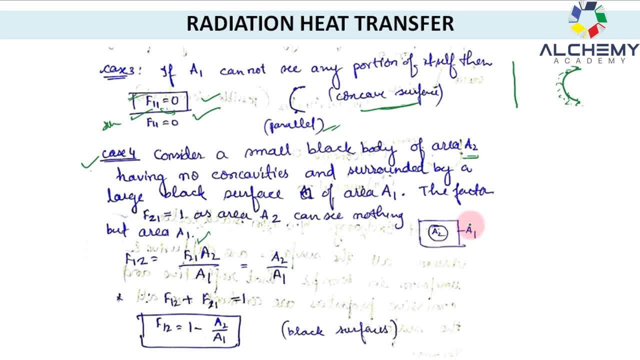 This is the body two. This is body one. Now, F of two. one means what? F of two. one means two is your source: amount of energy that is leaving from the body two, okay, and that is being intercepted by body A1. So A1, obviously it surrounds the body two. 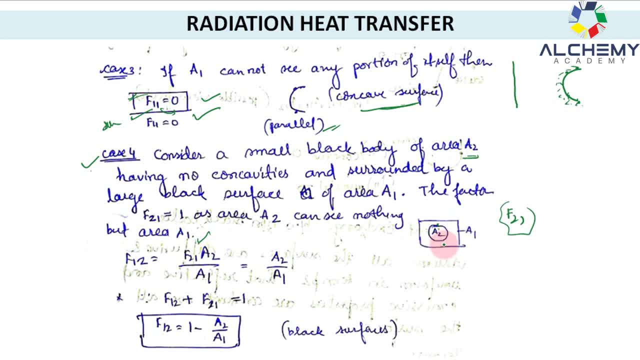 So it will intercept all the energy that is being, that is being that is leaving the surface two. So in that case, F of two, one would be one. So, as we know we have known earlier, F of one, two into A1, equal to F of two, one into A2.. 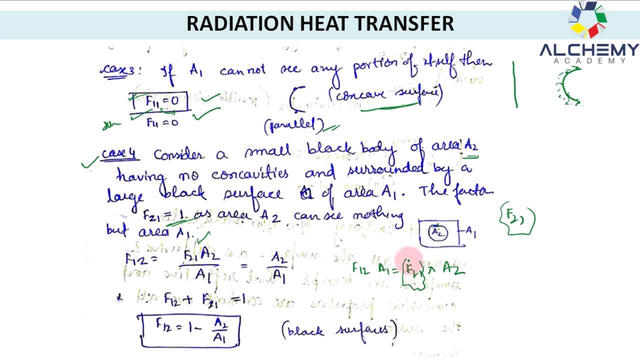 So in that case F of two one- we know that we have got an F of two- one is your one. So in that case F of one two becomes A2 by A1.. Now we see it here we got the value. F of one. two is equal to A2 by A1. 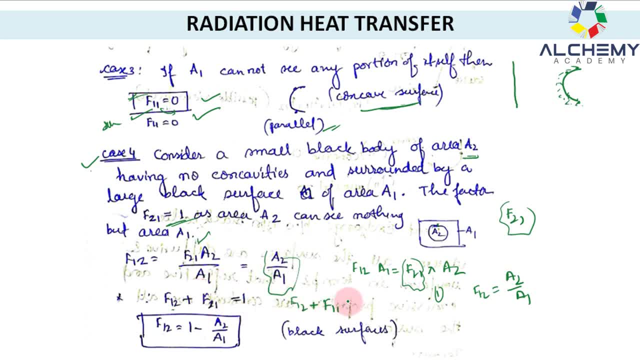 Now, as we know, F of one, two plus F of, since two bodies are there, is equal to one means. amount of energy- this is the one, is your source. amount of energy that is leaving surface, one intercepted by body. two and again, amount of energy that is being, you know, radiated leaving. 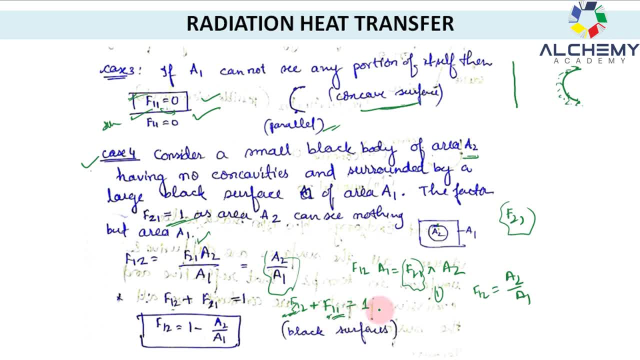 surface one. Again, it is being intercepted by body one. So in that case that is being intercepted by body two. So in that case that the sum of these two becomes one, then F of one, one equal to one minus F of one, two, correct? 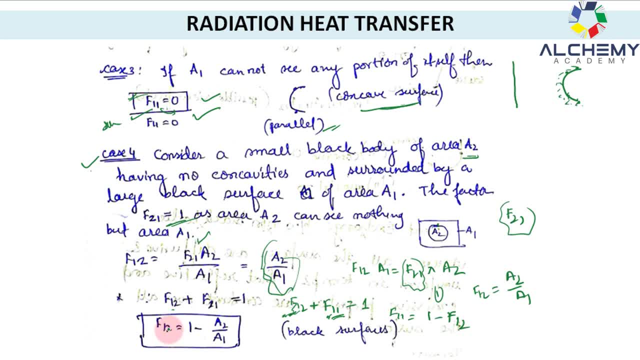 So, as we know the F of one two value, we know here A2 by A1.. So F of one two plus F of one, this is F of one one equal to one. then in that case, F of one two, F of one one is equal to one minus F of one two. 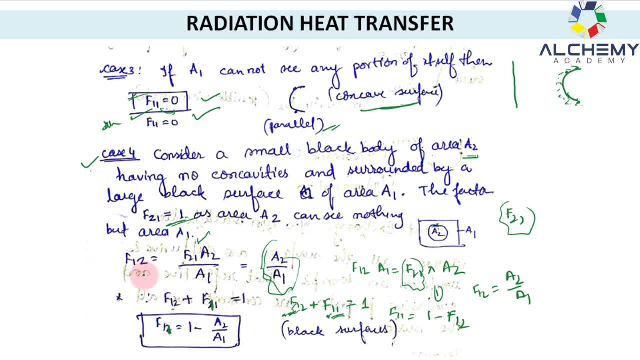 So this is: F of one one is equal to one minus F of one two. So let us put the value of F of one two, So value of F of one two is A2 by A1.. So we have kept it here, Correct. 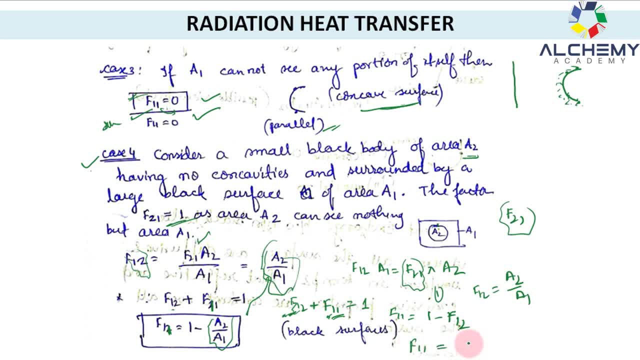 So that is why we have gotten the value F of one one is equal to one minus A2 by A1. Correct, So this is how we can calculate. So from this, you must remember this correlation: A1, F of one, two is equal to A2 into F of two. 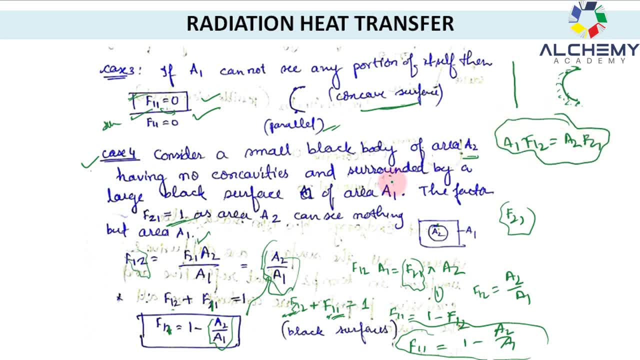 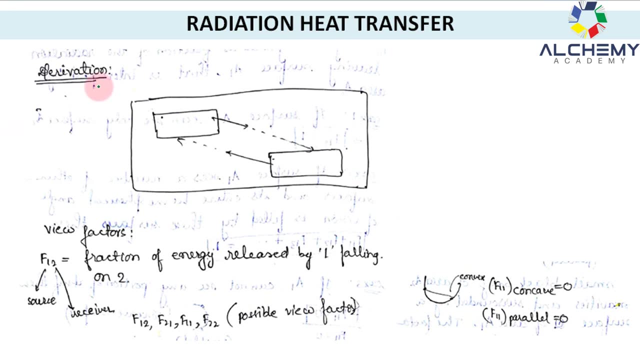 one Based on this correlation. many times questions has been asked in the GATE exam, So that is why I have told you these four cases to understand it clearly. Now let us see the derivation part: heat exchange between the bodies. for heat exchange between the bodies: 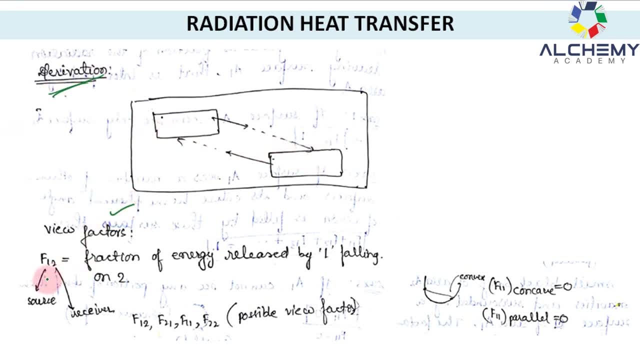 So this is the body one, body two, view factors, as we know. F of one is your, basically fraction of energy released by body one and falling on surface two means that is being intercepted by body two. Here, one is your source, amount that is leaving the surface. two is your receiver, which receives. 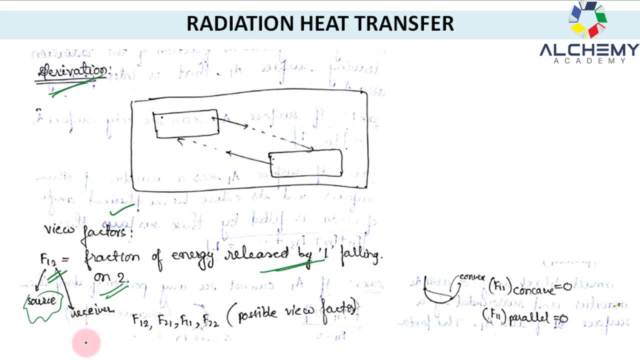 the amount of energy that has been. that intercepts the amount of energy that has been radiated or leave the surface. one. So this is F of one. So this is F of one. two, F of two. one, F of one. one F of two. two is the possible factor. 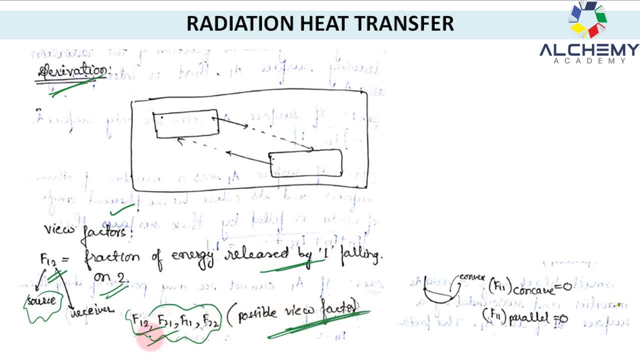 two bodies are there, then there are four possible factor. This is F of one, two, F of one one, F of two, one, F of two, two. Correct, Now suppose your parallel surface is there, then in that case what happens? our concave surface is there. 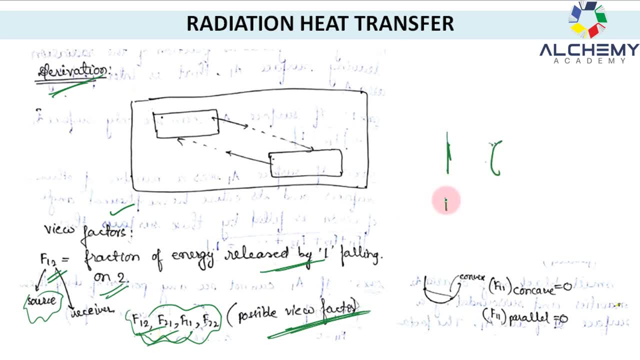 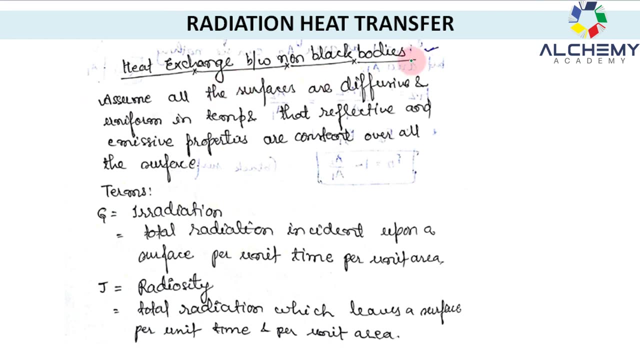 It would be able to see its own surface. in that case F of one one will be zero, and for this also, concave surface, also F of one one will be zero. So we must know the concept behind this. Now, heat exchange between non black bodies. now we will discuss heat exchange between: 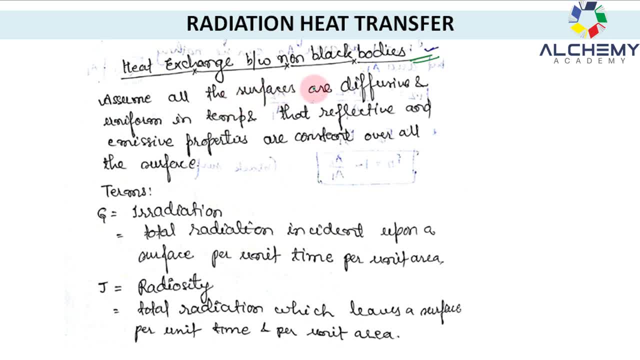 non black bodies. So let us assume all the surfaces are diffusive and uniform in temperature and that that is reflective and emissive properties. the reflective and the emissive properties are constant over all the surface. Now terms. we must know these two terms, G and J. 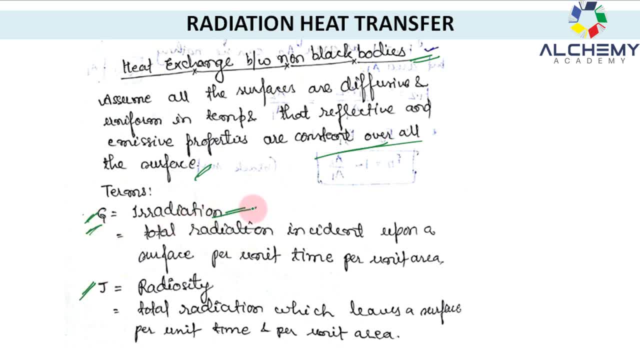 What is G? G is irradiation. So what is irradiation? It is basically total radiation incident upon a surface. per unit time, per unit area means incident radiation, total radiation. whatever the radiation, total radiation that is incident, incident on the surface, it is called as irradiation. 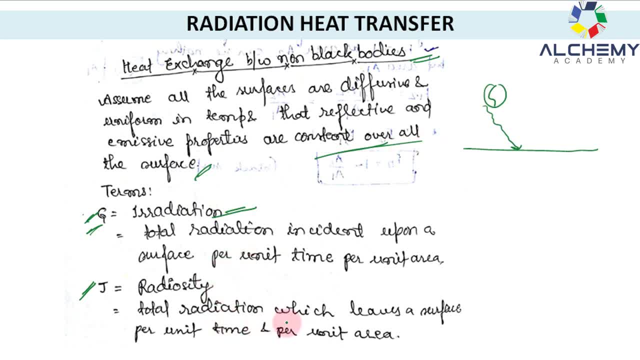 So this is G. Now what is the radiosity? total radiation which leaves the surface per unit time, per unit area. So the part of incident radiation obviously will be get irradiated. So G into part of that row, reflectivity, G into part of this is one and the second is 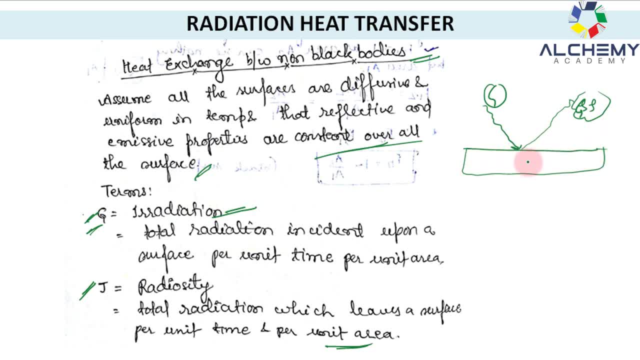 part the body will have, you know, the emissive property itself: It emits some radiation. Okay, that will also consider the reflective part plus emissive part of the body is basically your radiosity. So this is the total radiation which leaves the surface per unit time, per unit area. 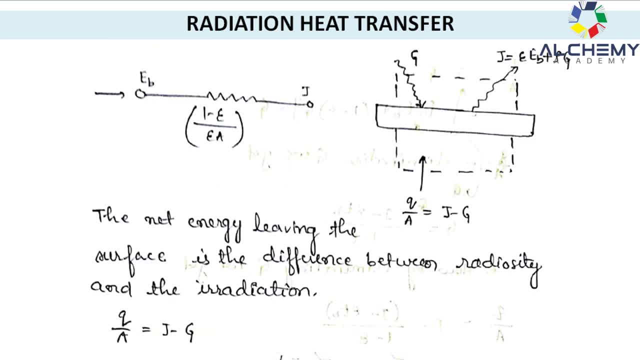 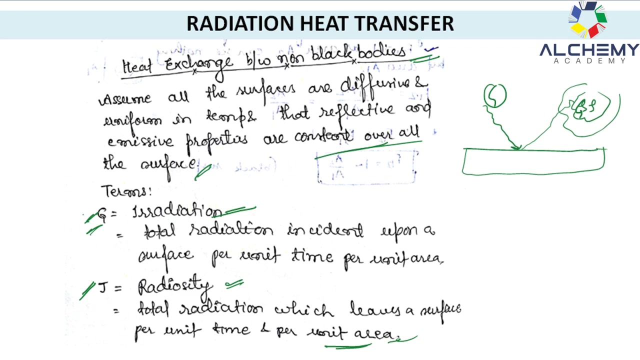 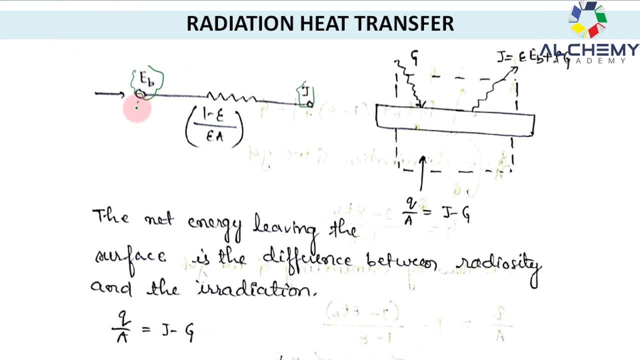 Now, this is AB, black body, This is G. Okay So, and this is the black body, energy here, G and this is G. This is your G is your radiosity total fraction which leaves the surface per unit time, per unit area. Now, net exchange between these two bodies, energy exchange between these two bodies, black. 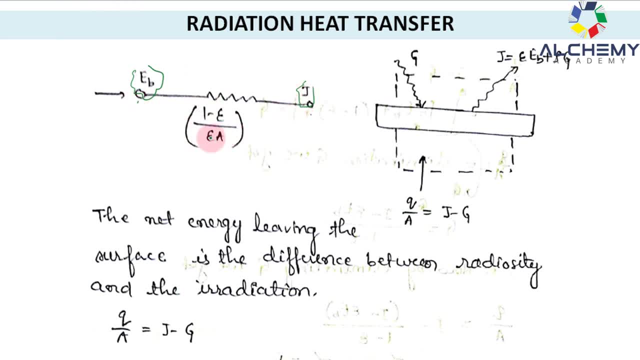 body and the non black body, E, B and G. This is your, basically one minus epsilon, divided by epsilon into A. This is basically the resistance. without any heat transfer happens because of the temperature gradient. Okay, Divided by the resistance, similar funda has been implicated, implemented here. 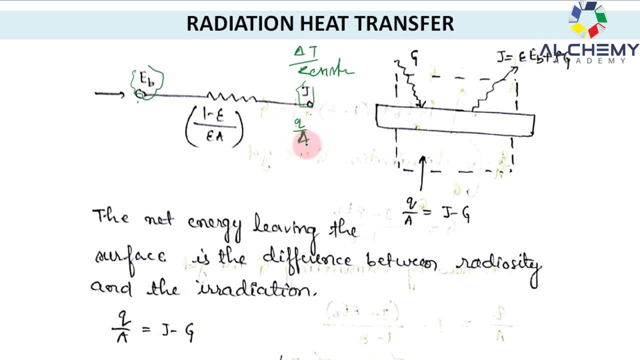 So here also Q by A would be like. I will derive this value what I want to say here it becomes it. well, it would be: value basically: delta T, delta T kind of equation, Exchange between the body, energy exchange between the body: E B minus G divided by its. 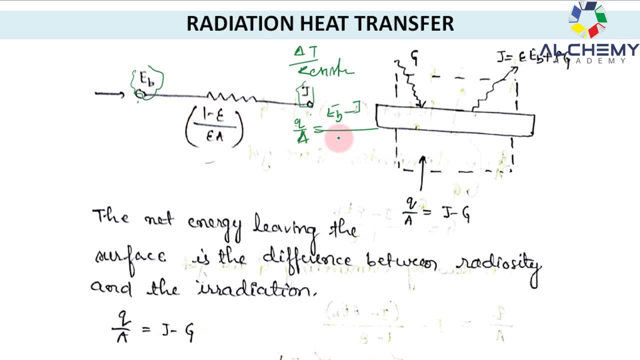 resistance, Resistance is- this is your resistance: one minus epsilon divided by epsilon into A. So this is the formula that we are going to describe from this. So G is your amount, of this is your irradiation. This is, that is what I have told you. 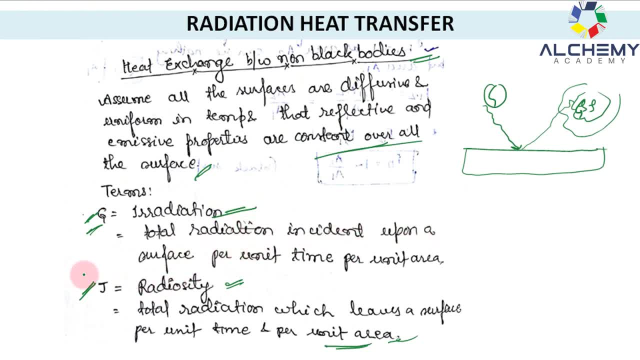 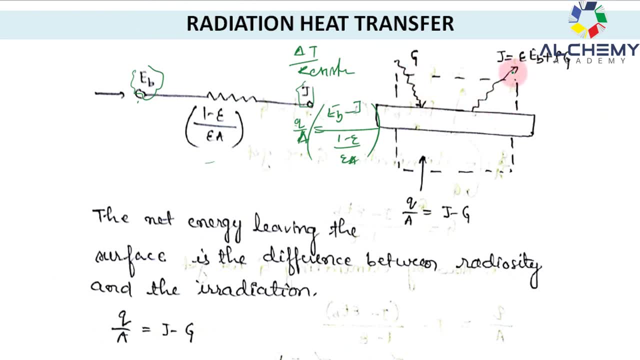 This is irradiation, total radiation incident upon a surface. Okay, So G is your irradiation And G is your radiosity amount of energy that leaves the surface. So E, B is your black body and emissivity, the power of emissivity. that E B is the energy. 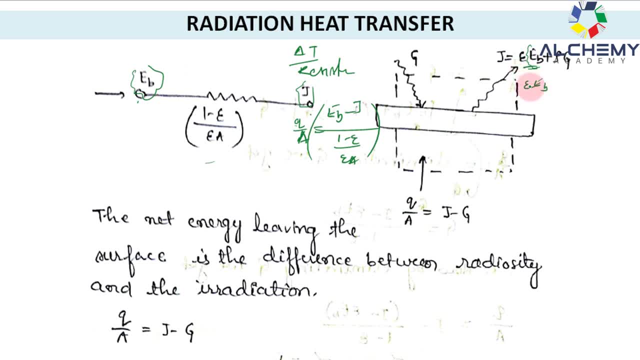 E, B, emissive power into emissive factor of that. So this is energy due to the emissive power of the body, emissivity, nature of the body and rho is your reflectivity. So G is the total radiation that incident upon the surface and part of that is being 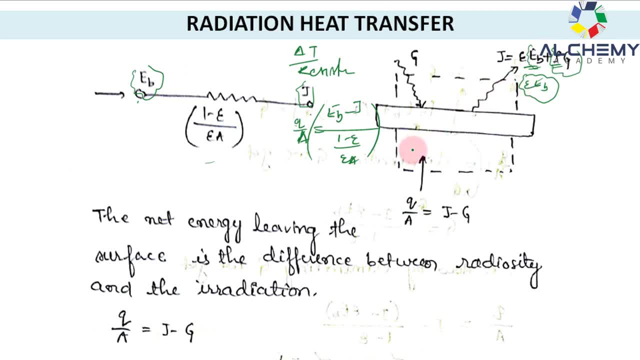 calculated that is termed as rho, into G, So Q by A. what is Q by A is basically G minus G. how much total the net energy leaving surface? Now we want to calculate net energy exchange between the bodies. So here it means that net energy that leaves the surface means how much energy is leaving. 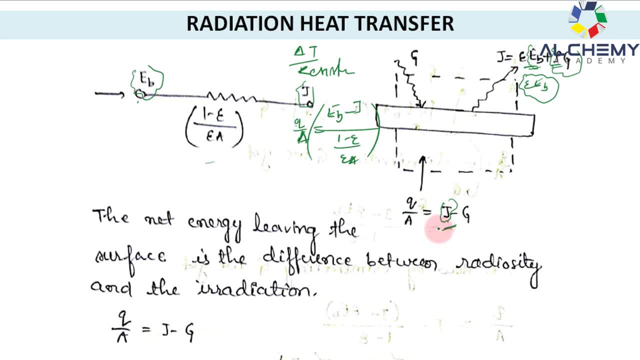 So this is basically G. G is the amount of energy that is being that is leaving the surface and G is your amount of radiation that is incident on the surface. G net on the surface, total radiation. So Q by A is equal to G minus G. 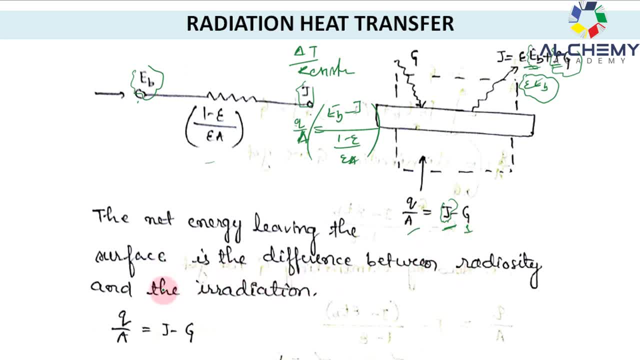 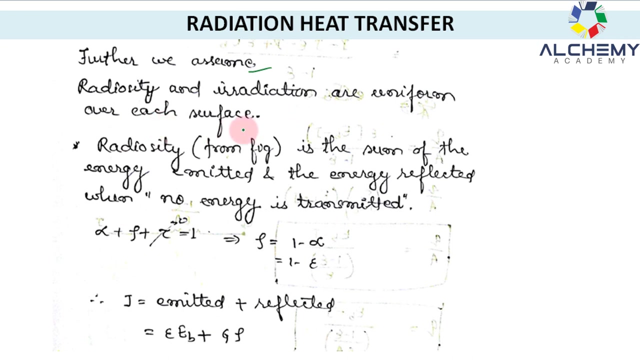 So surface is the diffusive between the radiosity and the net energy, leaving the surface is the difference between the radiosity and the irradiation. So this is the radiosity and the this is irradiation. Now further, we assume radiosity and irradiation are uniform over each surface. 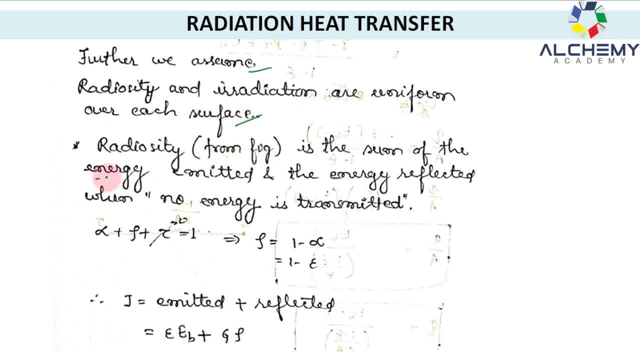 So radiosity is the sum of the energy emitted. So just see here: energy emitted and the energy reflected when no energy is transmitted, Correct? So when no energy is transmitted, So tau would be 0.. So alpha plus rho is equal to 1.. 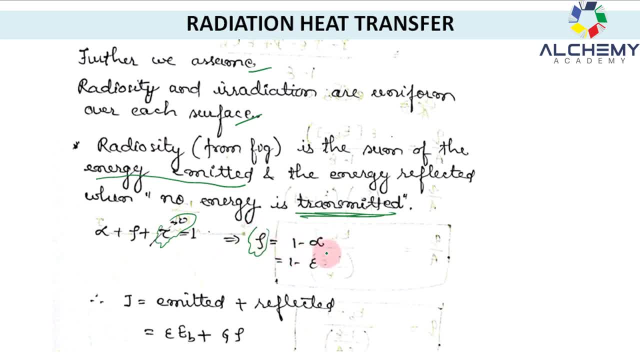 So rho becomes equal to 1 minus alpha. For black body, alpha reflectivity, you know, is equal to 0. So this is equal to emissivity. So we can replace this as here. So J is your, basically emitted, plus reflected is become epsilon to eb plus G into rho. 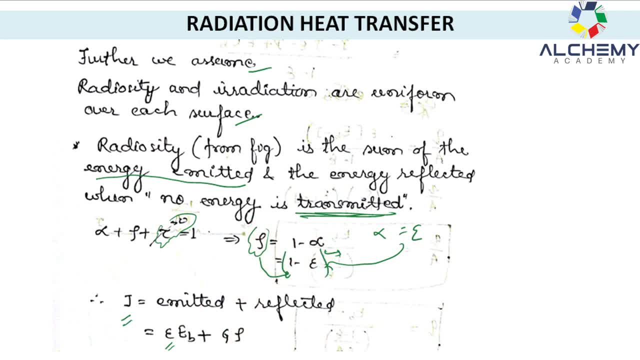 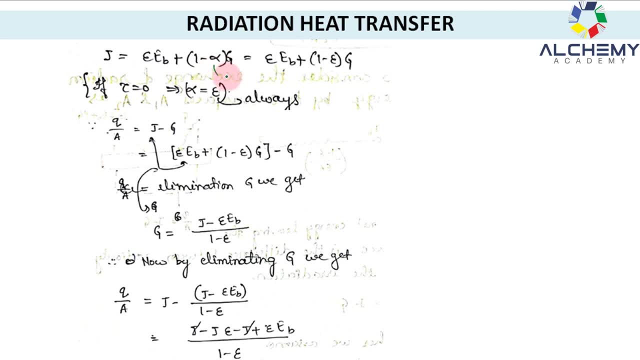 So rho value we can write from here: It becomes 1 minus epsilon. So let's write that. So J is equal to epsilon to eb plus 1 minus alpha into G. So alpha we can replace as from epsilon, So epsilon to eb plus 1 minus epsilon into G. 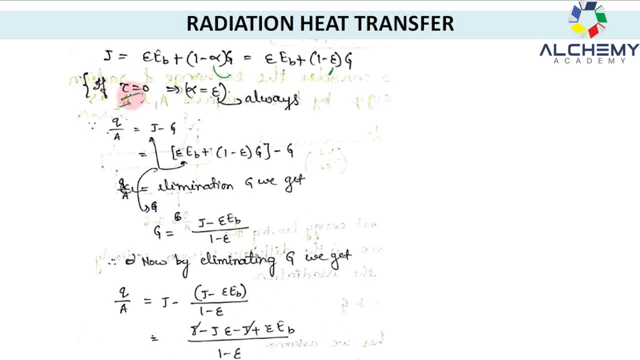 Now if transmittivity? If transmittivity is 0, then your absorptivity will be emissivity always. So cube by A is equal to J minus G. So J value, we know This is the J value Correct. So e epsilon to eb plus 1 minus epsilon into G minus of G, this value. 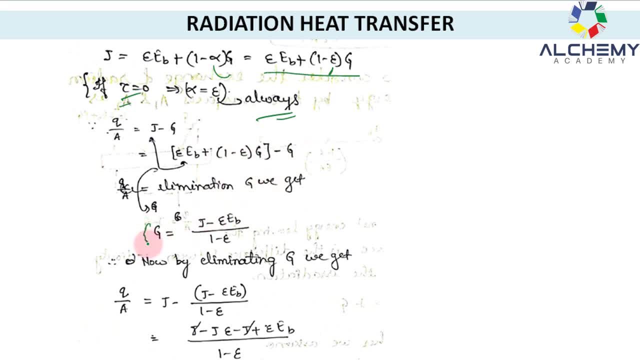 Now, if we eliminate, solve this, we will get the value of G as By J minus epsilon into eb divided by 1 minus epsilon, Correct, So this one is 1 and this is another equation. Now, if we solve this, from these two, we get the value of G. 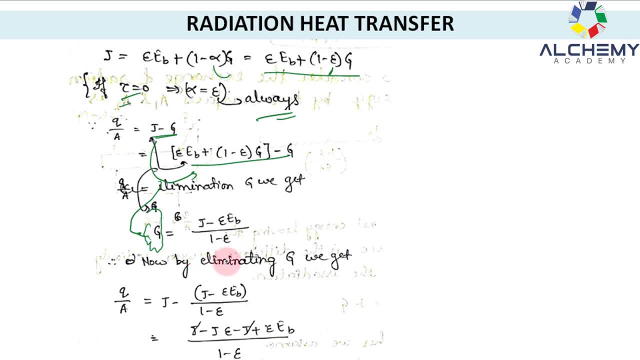 G is equal to J minus epsilon into eb divided by 1 minus epsilon. Now, by eliminating G, let's remove the value of G from where This What we will get: J minus this value, J minus epsilon into eb divided by 1 minus epsilon. 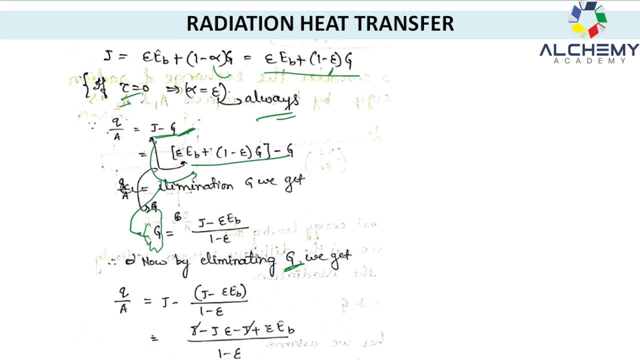 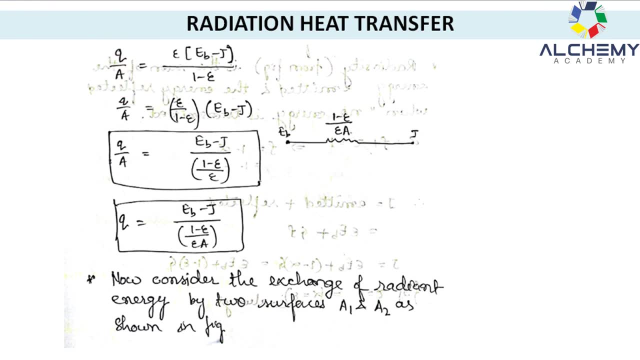 Now, if we solve it, we will get the value. We will get this value. Q by A is equal to epsilon into eb minus J divided by 1 minus epsilon. So Q by A becomes epsilon divided by 1 minus epsilon. take it in bracket- into eb minus J. 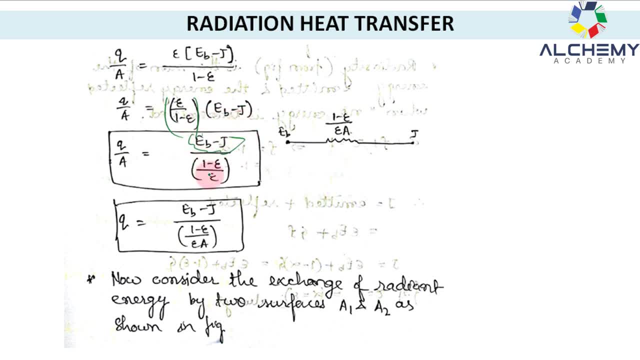 Now, if you write ab minus J divided by this becomes epsilon 1 minus epsilon divided by epsilon, Because this epsilon will come upside. So Q is equal to eb minus J divided by 1, minus epsilon, divided by epsilon into A. So this is the derivation that we wanted to tell you how we have gotten this, and you must remember.